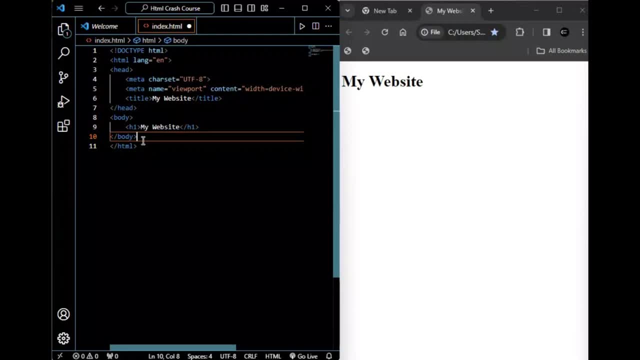 automatically All right with the opening tag, or we call that the anchor tag, and it closes with the closing tag, and most times- not most times, all times- it's. HTML 5 comes with that functionality, that the closing tag ends like this: Now an angular brace before slash and the name of the tag, then a closing of the angular brace. So that's how it's work with HTML and 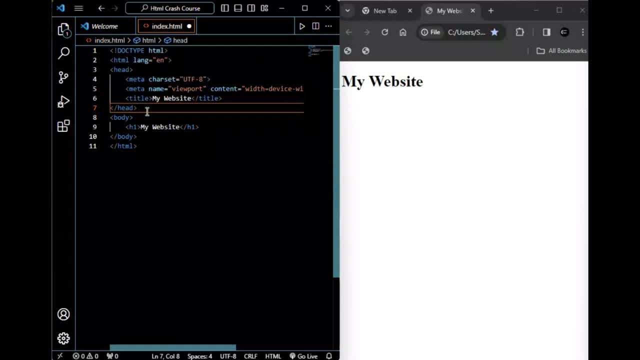 Next we have the semantic tag for the head section To go into semantic tag. So we have various tag that does various things in HTML and you see the opening at the closing tag is wrapped around the details or the, the, the details or the- whatever you want to display on on the web page. 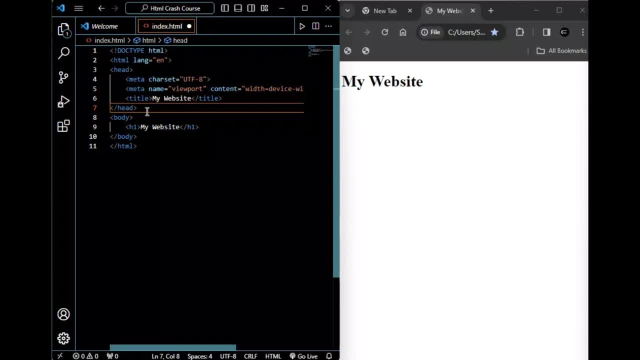 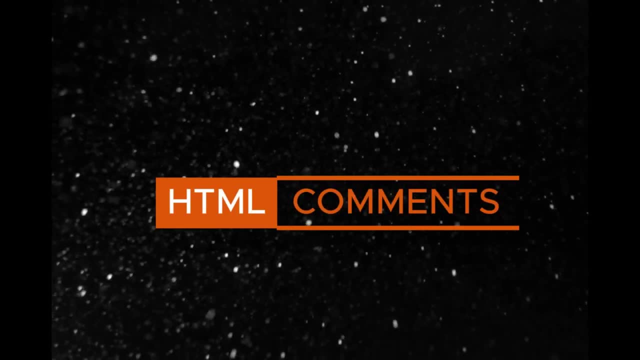 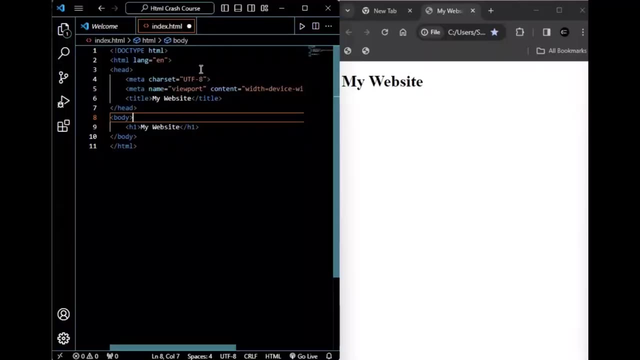 So HTML basically it's about giving right, and now you want your web page to be displayed, so we have what we call comment in html. so, for example, if i just decide to write uh headings here, if i save that and i reload this page, i'm going to, i'm going to see editing here. 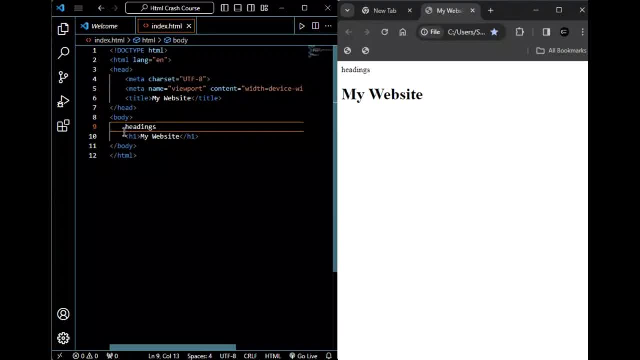 so what if i want to talk about this? i'll talk about what i'm, what i want to write now, without wanting it to show in my website. i just want to just have a comment section and just comment now. comment most times in program is about talking about what that line of code or the following: 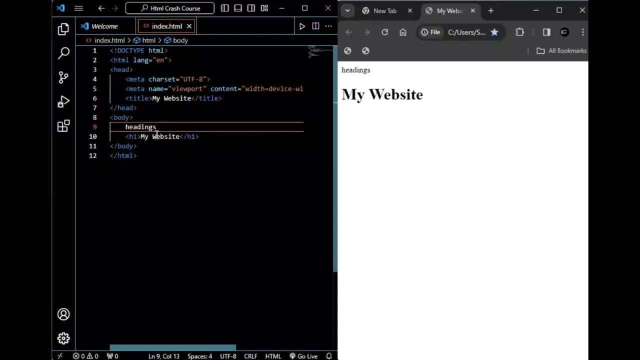 line of codes talking about, and, for example, what? let me give you an illustration. think so, this is an h1 tag, all right for my website, so i can come here and see. and how do you write your comments? it's very simple. you open an angular brace. yeah, so you have an apostrophe. then you have a. 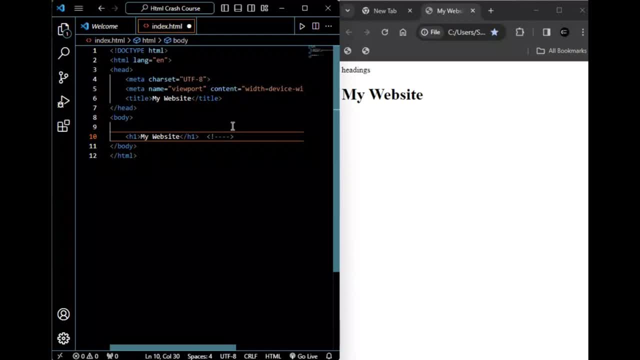 dash, dash, like this, then inside this, two things. okay, inside there you can have my tag so i can see: uh, let's see, i say this is the uh first header tag. all, right, now you can see that. so i save this. very load this. so i won't see this comment on the on the website, but it's just there for a comment. 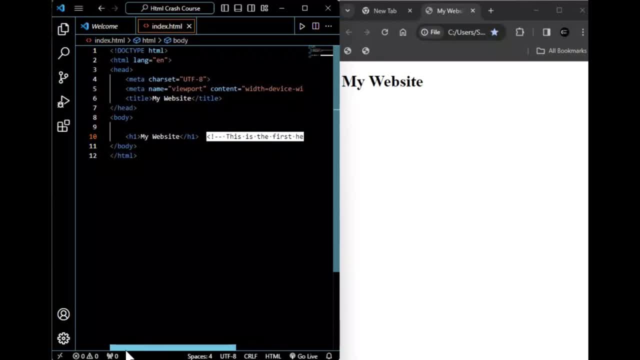 all right, so that let's say, for adventure, somebody comes to see my work, he knows what line 10 is talking about. so that's what comment basically is in computer programming and generally. let's clear all of these and just start with the semantic tag. we start with: uh, the doc type, the 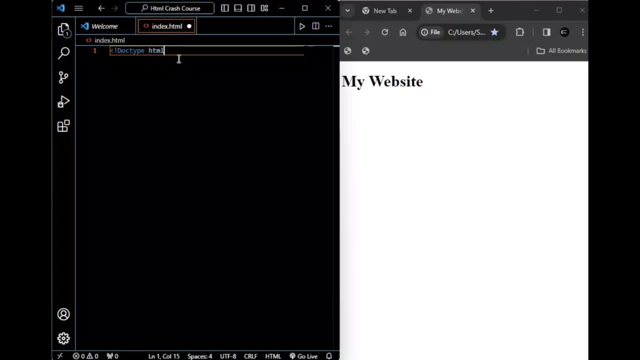 dark type html. all right, then you close that. then we have the html tag. so for vs code, or you can just write html and put it. click on your tab. it's the tab button. it's going to complete it for you. so inside html we have the. 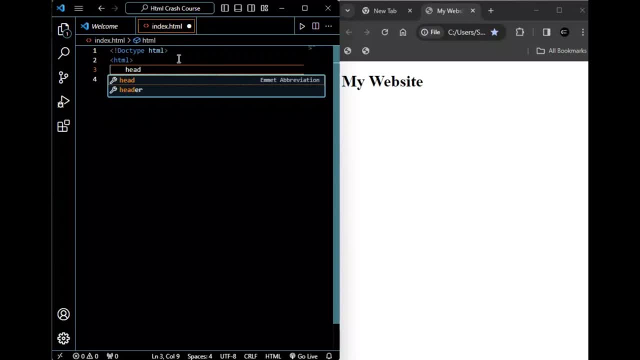 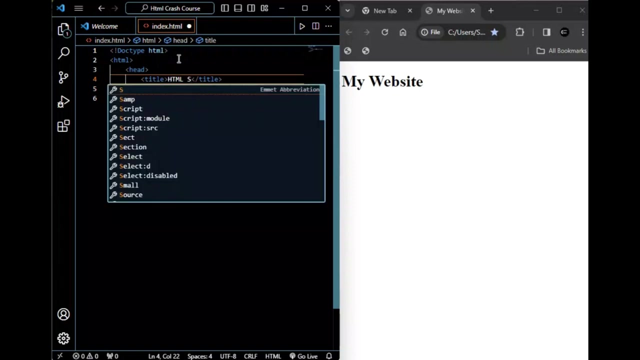 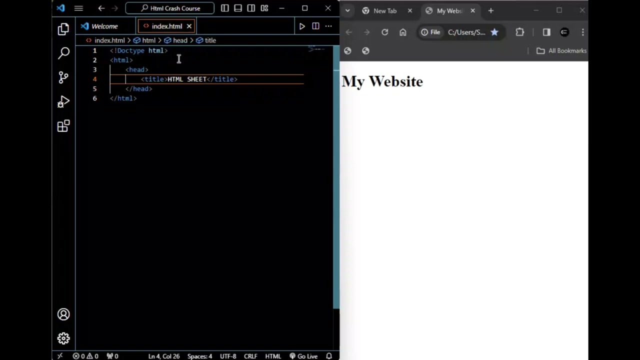 edge session. just write edge and tab, and inside the edge session we have the title: yeah, title. so what should we call the title? let's call the title now. let's call it html, html sheet. all right, so we save that and reload this. we shall have the html sheet. and before we go on, let me quickly show you a cheat. 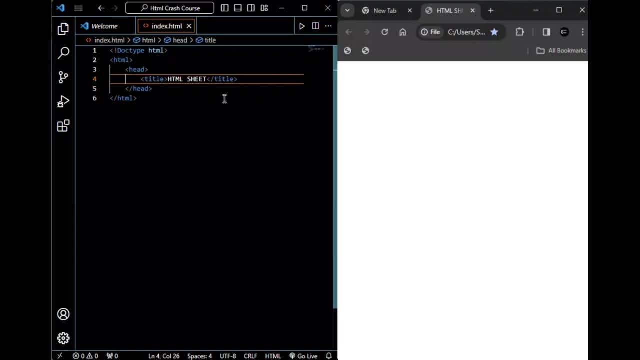 try, say, cheat or a plugin, all right, in vs code that makes, uh, this, your coding more faster and easier, you? so you come here. this is an extension, all right. so you click on the extension. you come here and search for live server. so you see your live server. you click on the live server. 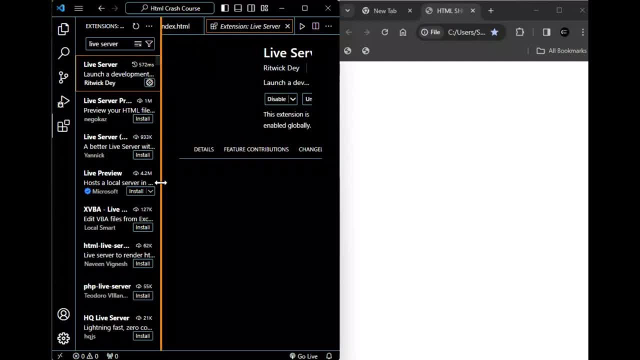 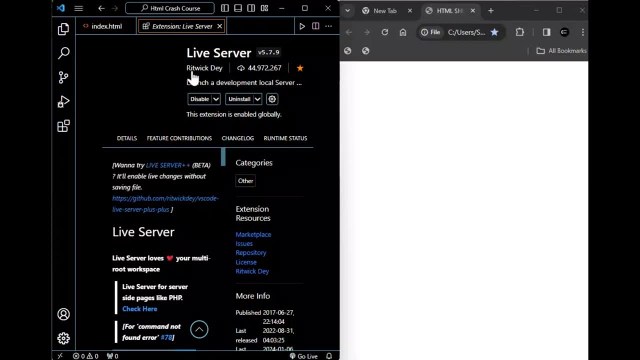 now you are going to see something like this. let me close this tab. so i'm going to do something like this: a live server like this, yeah, by a weekday, and uh, i already have it installed. so if you don't have installed- of course, if you are just going through this, you will- it will not be installed. so you're going to. 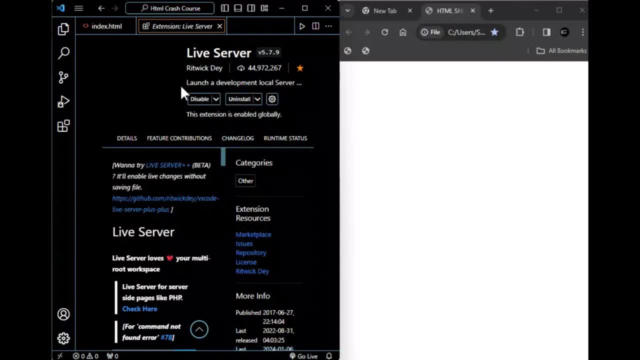 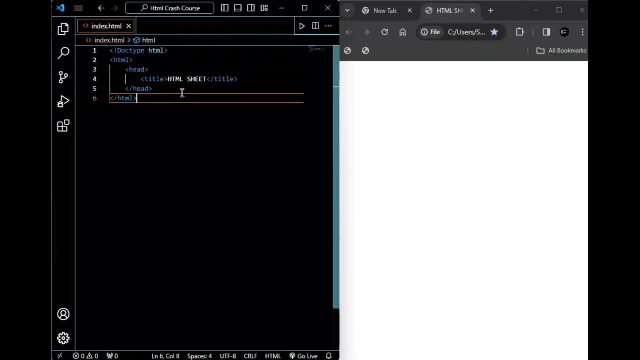 click on install and this is going to install your computer and i haven't done that. you can return back. you can play this and return back to your html sheet. then you see something uh down here and that's go live. when you, when you click on go live, so it will start and uh all will. 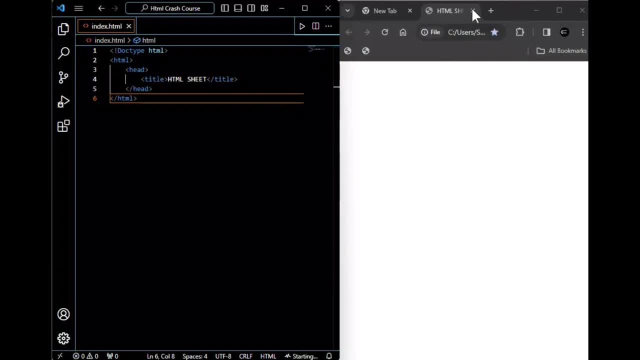 happen is that on my browser is going to create, uh, another, uh, another tab. all right for a. okay, i'm just going to do that now, just take some time. and you got to create that right here you can see. so you can see that i have it, have a port number and that's going to be for this uh code. 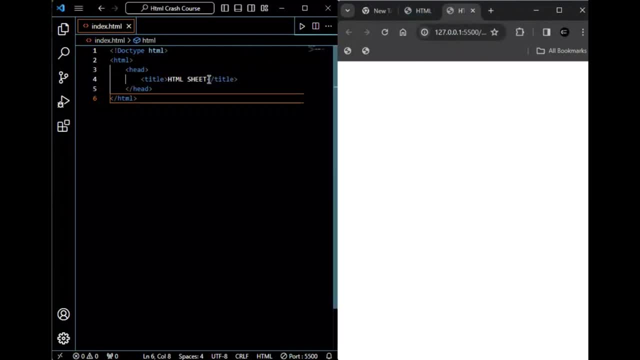 all right, and you can see it now. what i need to do is now, if i, if i decide to let me, let me take with this, all right, and this, now this html sheet. so let i say i say html, i say book sheet, all right, and i save this, it automatically change. you can see that without reloading it. so it's. 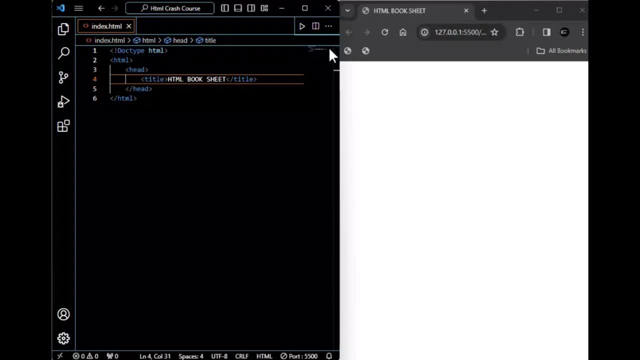 automatically uh change on the browser and that's the work of that extension, all right, so now let's have the body. so have the body, all right, and this way all uh tag is going to go. so i want to talk about tags. so the first tag we have is the heading tag. 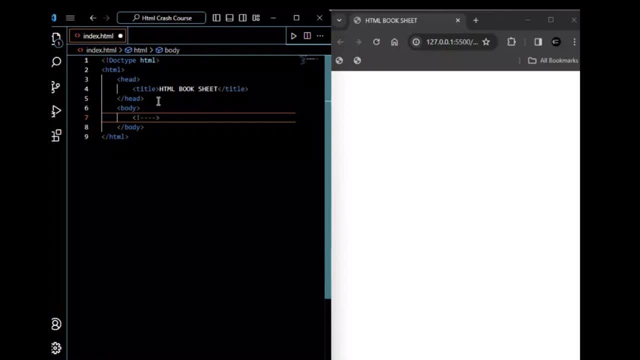 and i'm going to just pin that down with the comment so that uh can actually uh see heading tags. so under this session we have uh six of them. i'm just going to rush through it. so we have, um, the h1 to h6 and you know, the the. they already padded, at least to the basic. 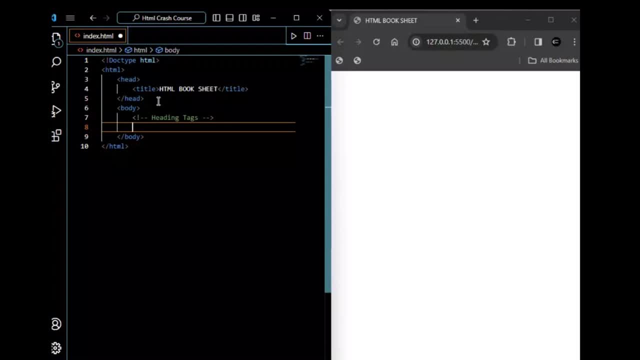 structure of uh, of of the headings, all right. so what we should have, of course you're going to- can't see manipulate with that, with uh, the css, but in this training is just going to be html, strictly, all right. and we're going to have another series of css, all right. so let's start from h1. so i say h1. 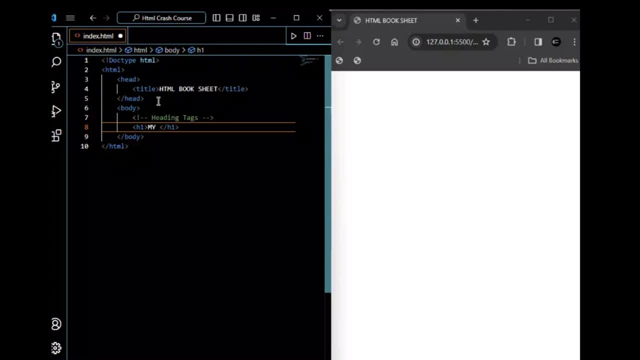 and it's not h1. i say my, uh, my ending one. now i save that. see that my editing one is, uh, the big. all right, that's a big font and it's bold. very good, so we have h2. let's call that my editing two. 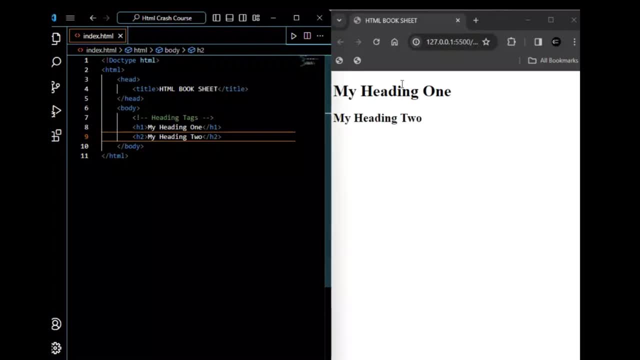 all right, save that, we'll have it. you can see it? not as big as the editing one, it's quite smaller. that's the heading two. so when you just copy this and, uh, copy that, so i'm going to copy that and paste that, so i'm just going to change. 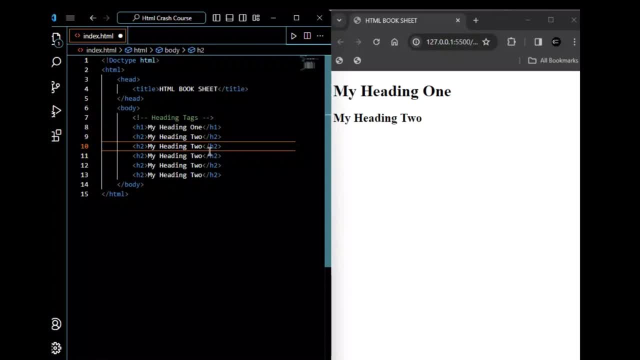 it. so i'm going to come here and change this to three. all right, so i'm going to change this to four. okay, four, five, six. it's gonna be six and this is going to be five. i'm going to change this to, uh, three of this. 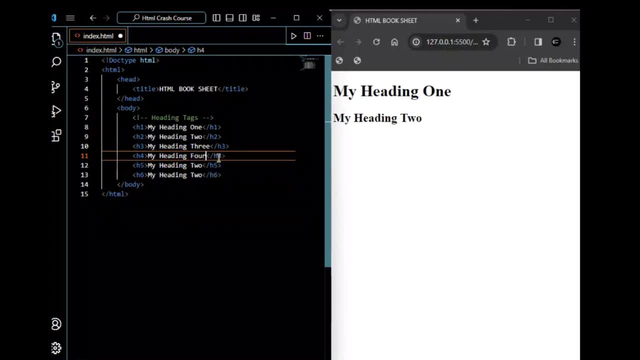 to be four, of this to be, i think, five. i'll have this to be three, six. all right, so we save that. you can see we are from the first editing to the last study. it is formatted according to the- uh, the structure of the html5 semantic tag, so we have it like that. 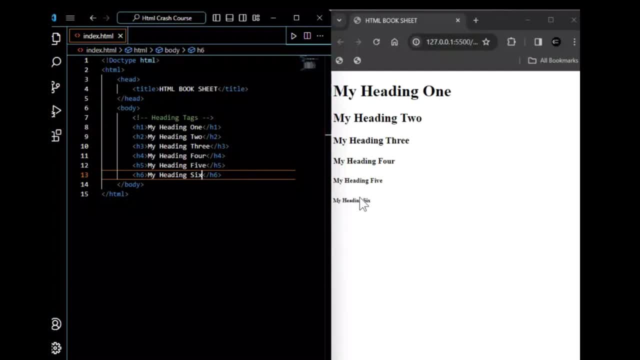 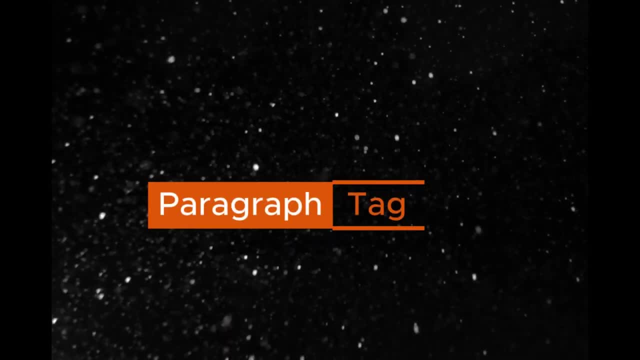 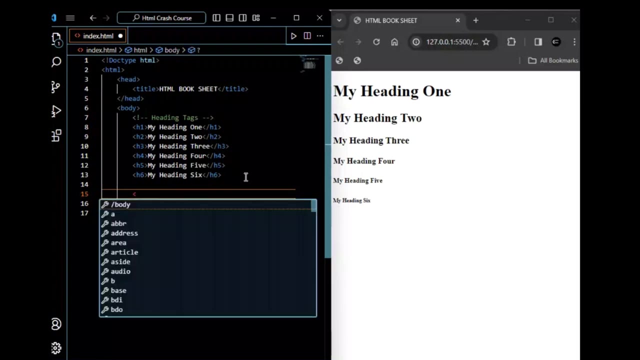 and most you use them according to how you want to use them. so i'm just going to show you the basic syntax of how tag work and it how it's been structured in html: the paragraph, the paragraph text. all right, so i don't have a comment for that. let's say: 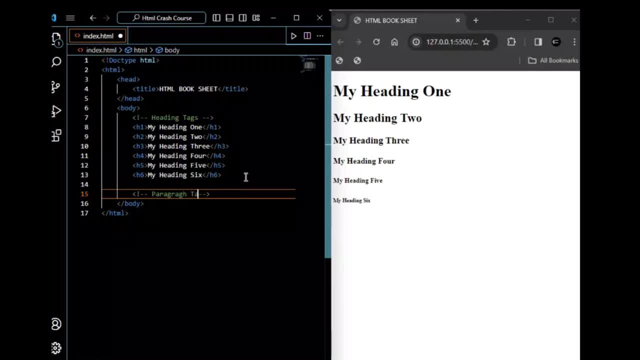 paragraph. all right, so how does that work? paragraph tag is represented with the p letter p, so you have just uh, opening and closing right, and your content, your paragraph, is going to be between these in in a vs code and many other editors. there's something you can do to generate a domain. 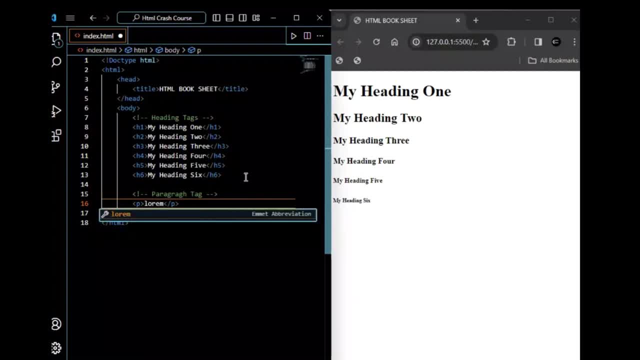 paragraph. all right, that works, just see lorem. and you just hit the tab button, it's going to complete with a full paragraph, so you can see that at a full paragraph. let me just close it, the full paragraph, and you can actually decide. select by. save this, so you can see. 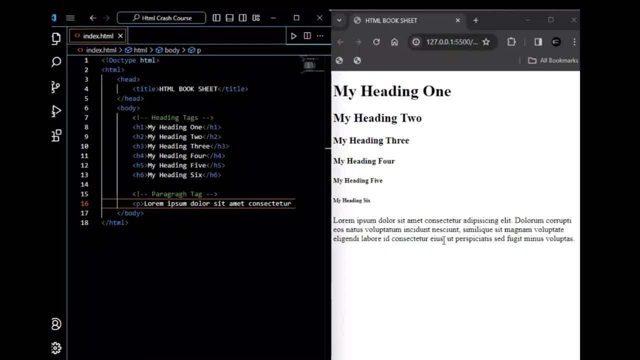 a have a paragraph. it is auto padded, auto margined, based on the basic margins and paddings of paragraphs. so we're not going to go into parties and margins now. all right, not in this video. all right, probably in the next in the css uh series, right, but in this series that's going. 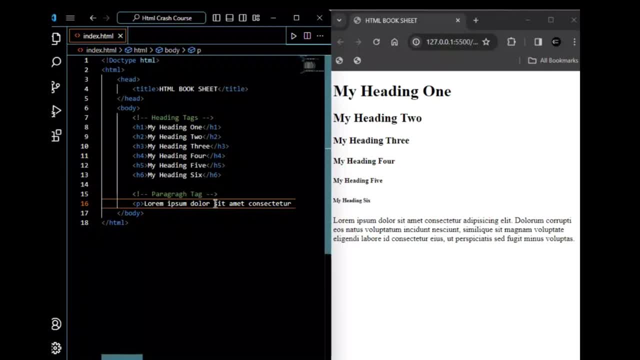 to be on html alone, but this is how the paragraph is being structured. and there's one more thing i want to show you here. you can see your lorem and you can see lorem 35. so you're going to hit the tab button to generate five words. so you can see. 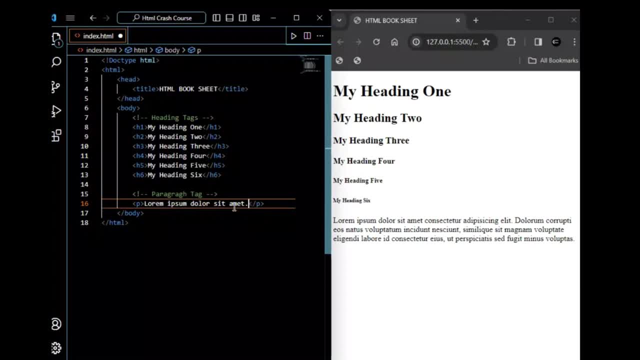 lorem and all of that. this- i think this should be spanish word- generate five of them. all right, so you can see that, so you can generate as much as possible and specify depending on the length of what you want. so that's about the paragraph tag, so i'm going to say the hyperlink. 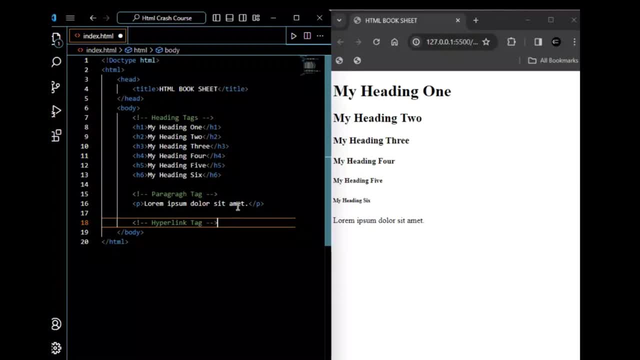 okay, hyperlink tag. okay. so let's have a paragraph. okay, let's see, let's say lorem, just 15.. all right, now i created a paragraph because, when it comes to the hyperlink, the hyperlink tag is an inline tag. all right, so what's an inline tag? so we have two. 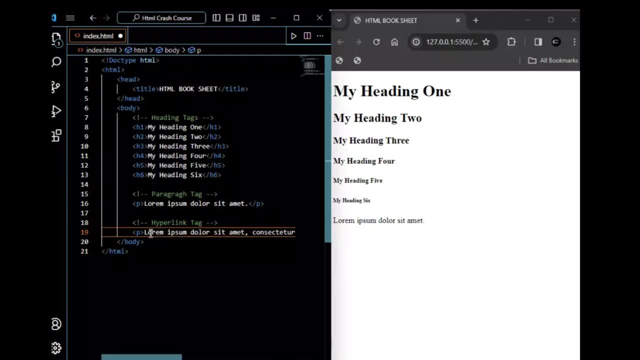 two types of html elements. we have the inline and we have the block. okay, so the block elements are elements that actually begins on a new page like this, on a new line. rather so we can, we we always have them on the new line. they start a new line. 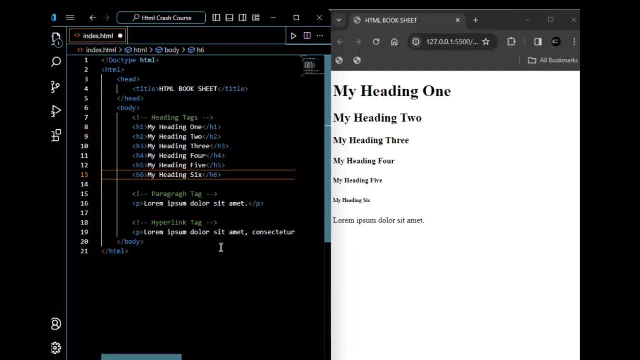 but an inline element most of the time. work on uh, a line already. for example, let's say i want to make uh, let me save this now. i want to make, i want to have a link, i want to make this word, this. i made all right this word here. i want to make it a link now to make it clickable. 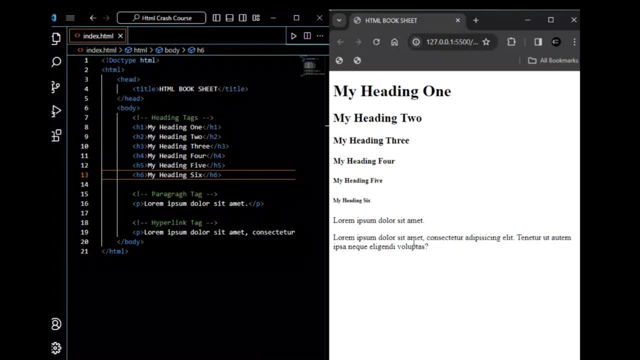 i'll make it clickable. so what do i do to make that clickable or to wrap a link around that? so all i need to do is to use the hyperlink tag and look for the the word. here. it is the word amit, and all i need to do is just to have it is represented with the a tag. 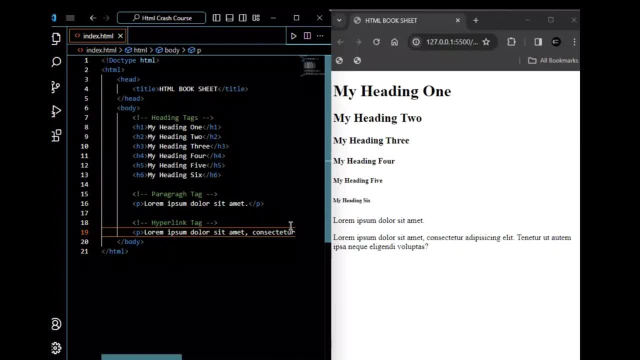 so i open it up. i have an opening tag and i say the a tag, all right, all right, and i close it here. i close it here now. this will not work because the hyperlink tag needs to work with an attribute. i want- i'm going to talk about that shortly- what an attribute is a tag attribute? so let's. 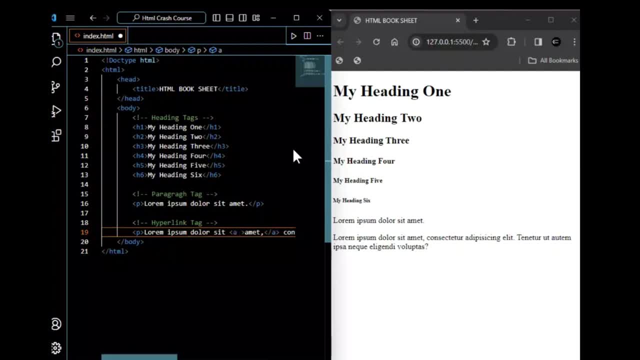 add an attribute to make it work. an attribute is just, uh, having to talk about giving a functionality to how the tag is going to work. so we have different attributes for different tags. so we have attributes. let's first we're going to use the href attribute. i'm going to explain this. 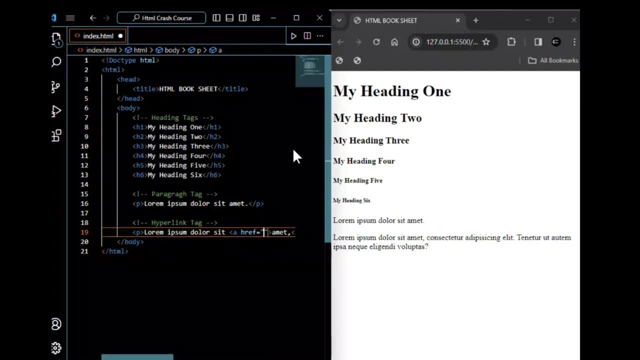 in a moment. now we have the href attribute and these attributes. now, since we are wrapping amit in a link, all right, so we're going to specify where we want this link to take in the visitors to. so we say: take them to googlecom, for example. so i say https. 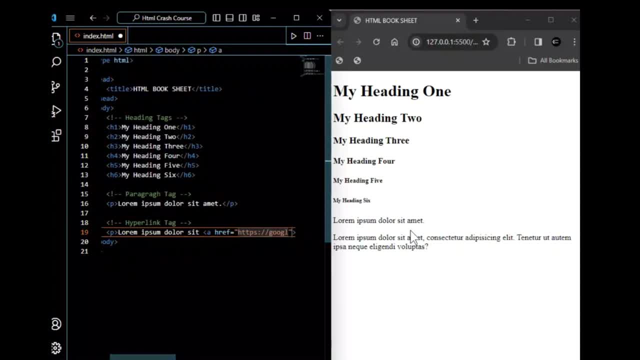 all right, and i say google, googlecom, all right, if i save this, you can see that. and this is wrap. the amit is wrapped inside the hyper hyperlink tag, so i saved that color changed to the default color for links. that's purple and you can see anytime my cursor goes close to it. it looks it, it, it. it changed to. 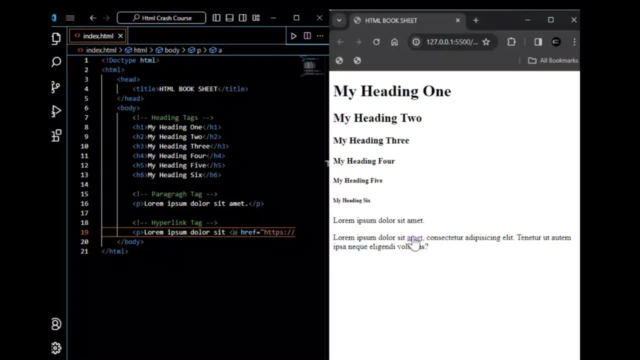 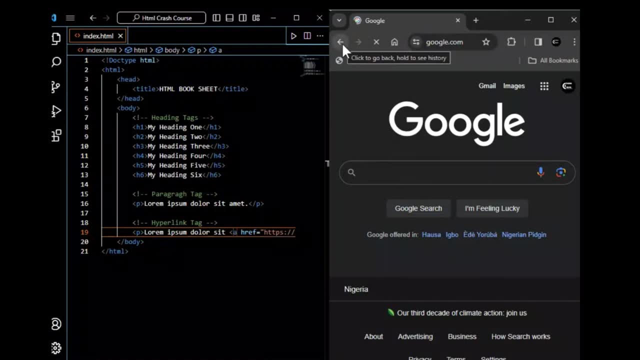 it look clickable. so if i click on this link now, let's click on and see, let's if it's going to take us to google. you can see that when google brought us google. but what if i don't want to to leave the current page? all right, i just want the link to take the visitors to another page. but 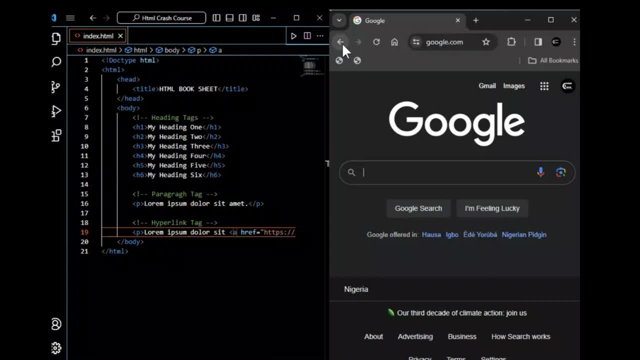 still maintain the page that the visitor is currently, so he's also just going to open the new page on another tab. so what i'm going to do is to add a page on that page and paste it into the home page now. and I told you that href attribute will be put in here, so we need to make that move. 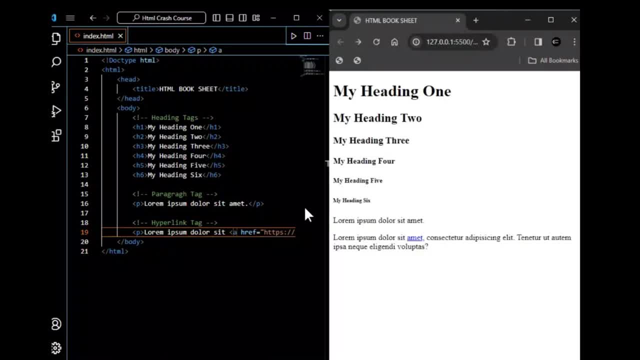 tab. so all i need to do is to add another attribute. to do that, let's go back. so i come here and, uh, i add another attribute. okay, so the first attribute i add is the href: just reference the location of where i want the link to take the visitors to. next is to, uh, have another attribute. 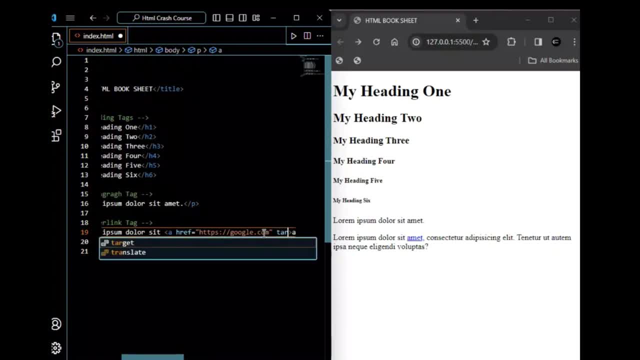 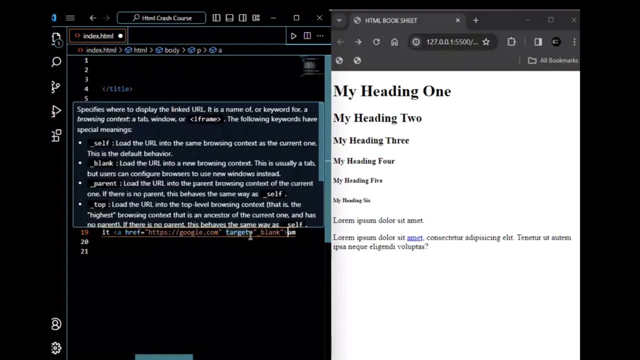 called uh the target. i'm going to say target and uh inside the target. i'm going to have an underscore blank. so this attribute will allow uh, this link to take. people visit us to googlecom on another tab on my browser. so let me save this. if i save that, all right, let me click on the link now. 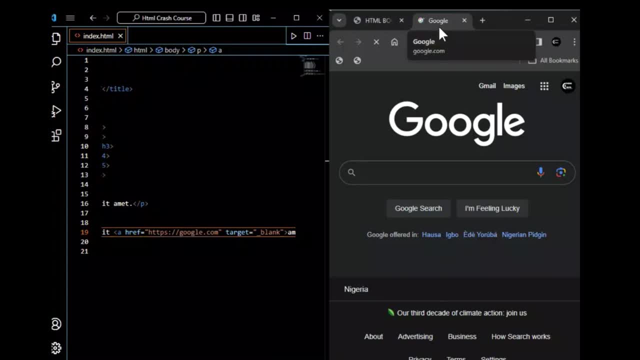 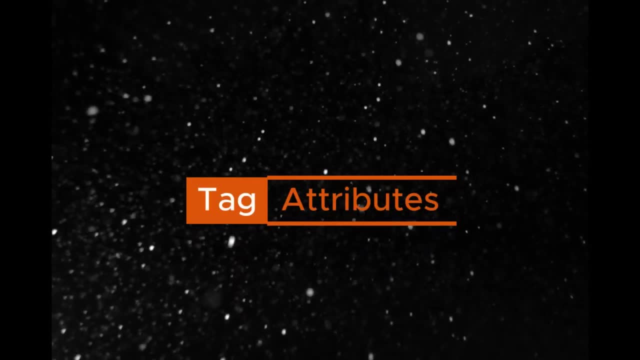 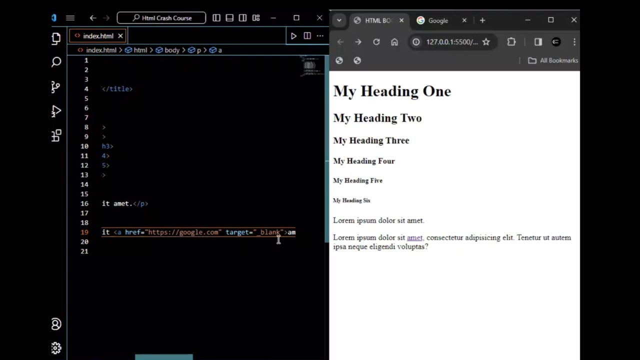 and let's see what happens. so we see that you can see googlecom opens on another tab. so that's just the so what are attributes? html attributes? the attributes are elements that determines the kind of assignment or the nature of the assignment of the tag. so it's always inside the opening tag. 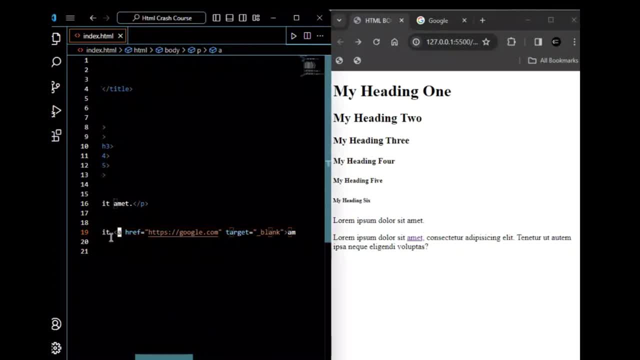 now i said this is the opening tag. the opening tag is time for the hyperlink tag and attribute. the first attribute you have is the href and you can see it's inside the opening tag. now what are the things actually work with an attribute? so an attribute is always written like this, so href in. 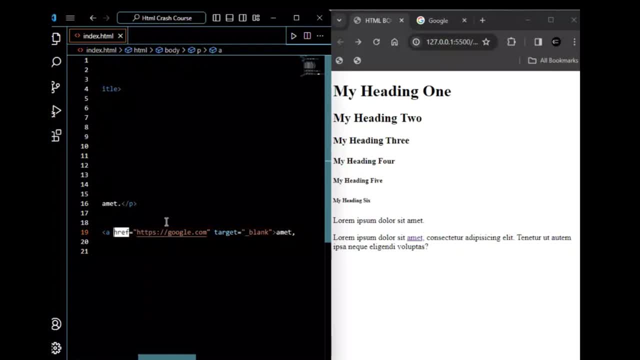 this sense is the attribute name. all right, href is the attribute name and the what does href do? and i just explained that href allows you to uh insert the url you want this link to take people to. so that's what this href attributes do and the target attributes. i explained earlier that. 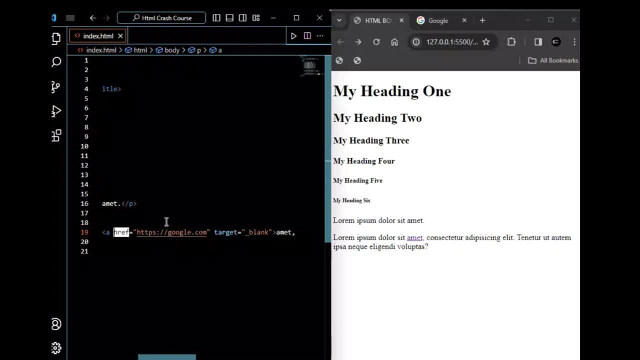 the target attributes, especially when it's selected as blank. it takes people to another tab, opens another tab with the link, opens the link, the url on another tab. href in this sense is the attribute name. target is: this is the attribute. you can see that in our code editor, the color is blue and so that you can actually identify it. 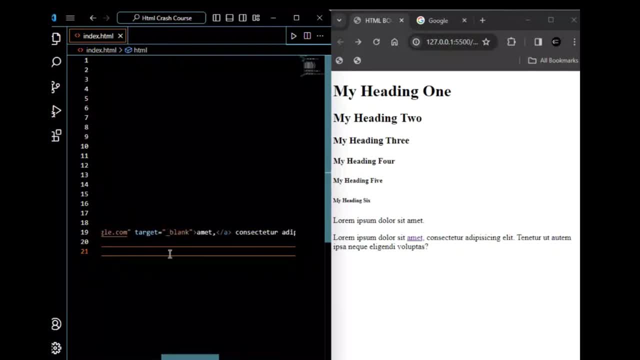 okay, an equal sign. so we see an equal sign and a double quotes and inside the book we have the attribute value. so target is the attribute name and blank is the attribute value. the same way, href is the attribute name and https- googlecom- is the attribute value. 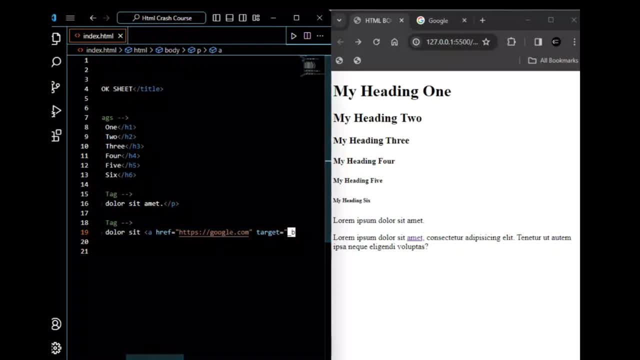 all right, so that's that about uh hd match. so we're going to use many attributes with many tags, and don't forget that attributes are always inside the opening tag.